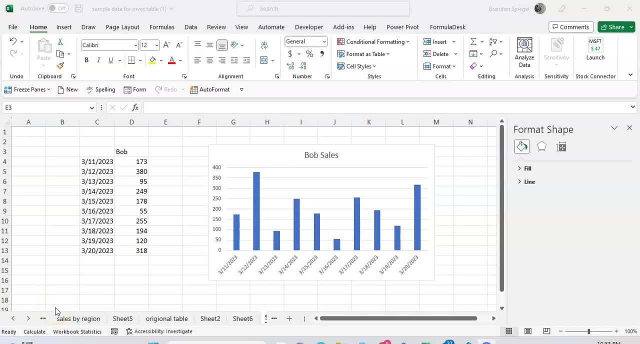 Hey, what's going on YouTube? I just wanted to make a tutorial to show you a cool trick that will allow you to have a different color to highlight the maximum value for a bar chart in Excel and then another color that will highlight the minimum value for a bar chart in Excel. 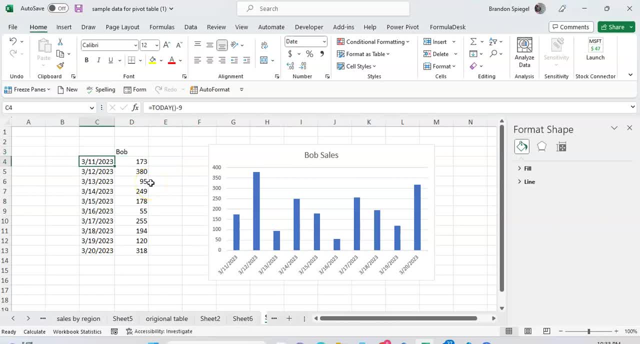 So here we have just a basic bar chart- Bob- what were his sales for these 10 days? And we want to have all the bars are blue now, but we want to have a different color for the maximum and another color from the minimum. So to do this, first we are going to make a new column called min. 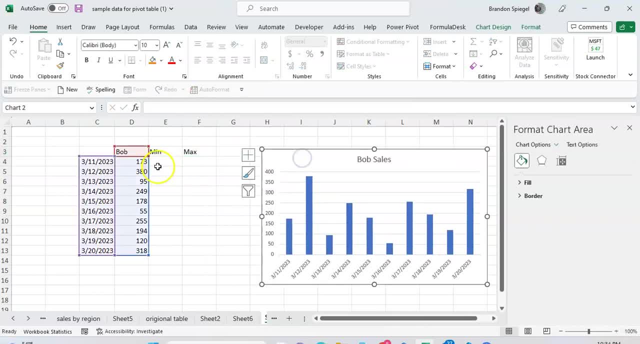 another called max. Now, with any of these columns we're going to do, is you're going to write a formula that says, okay, if this cell right here is the minimum of this range, then it's going to return the minimum. If not, it's going to return an A. 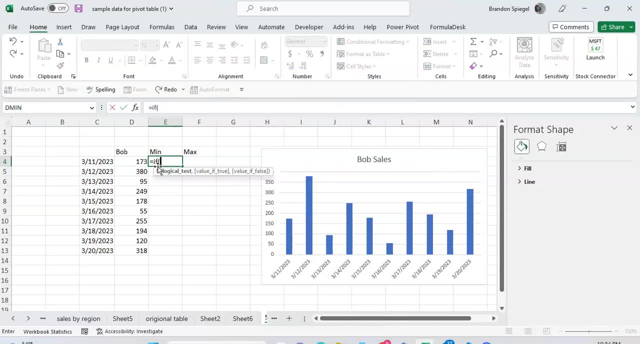 So did you do this? this do equals. if this equals the minimum of this range, the value for true would be this range. but if it's not the minimum, then just return na. and the reason why it's na is because of na, whenever graphs on the chart will just show up as blank. so that's why. 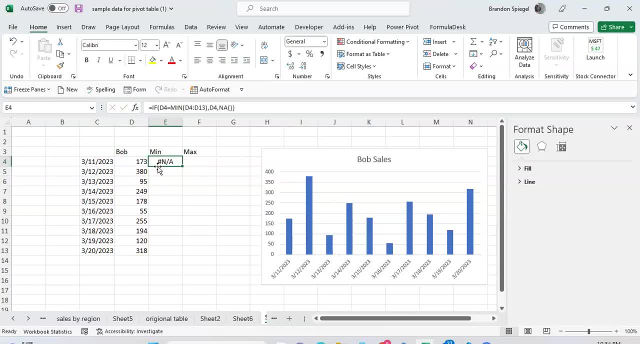 it's na Now, as you can see, this is not the minimum, so it returns na. but if we're going into the solid itself, locking these down, so function f4, because I'm on a laptop, we're f4, if 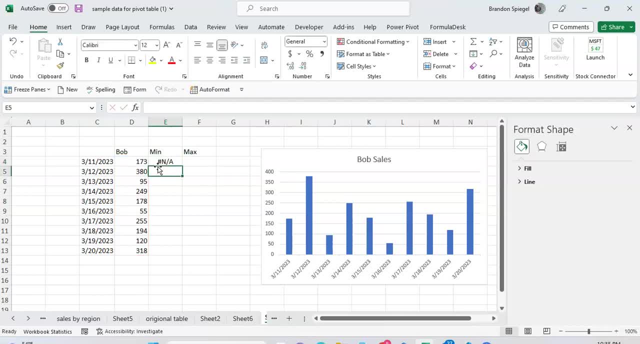 we're on a PC locking this down, to lock the range, highlighting this down and, as you can see, everything is na except for the min. Now we're going to do the same thing for the max, so copy and paste this over. 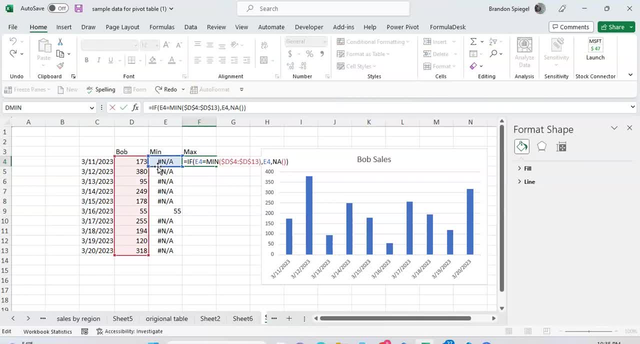 Going into this, going into the formula now, adjusting the little blue boxes to be in the right column and changing the min function to the max Control c and then placing that down and, as you can see, it does the same thing for. 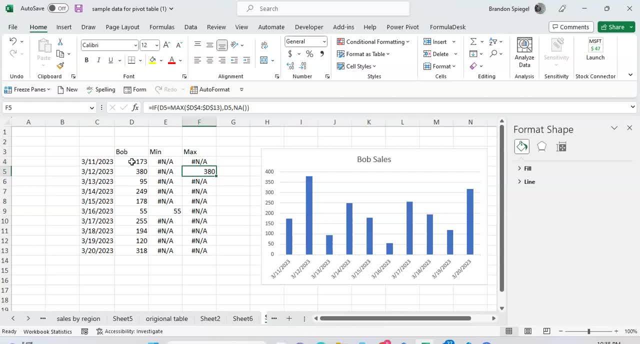 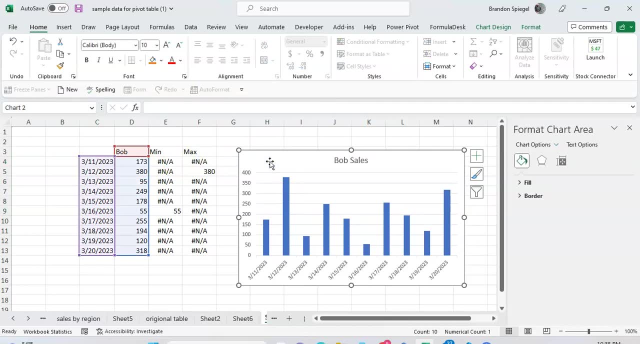 the max, but there is only the max value, which is 380 for the range, and everything else is na. Now, what we're going to do with this is we're going to get this bar chart, make it a clustered bar chart and then adjust the series overlap so that way the series appear to be one and 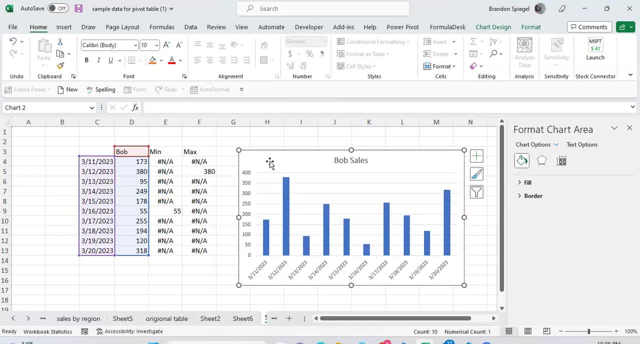 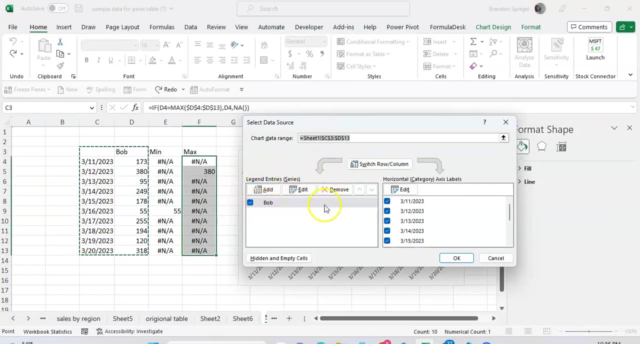 then it kind of gives a visual effect of highlighting the maximum or the minimum bar. So to do this, we're going to first add the new ranges that we just made. so click on the little filter icon, click select data. As you can see, right now there's only one range selected. we're going to add a new range. 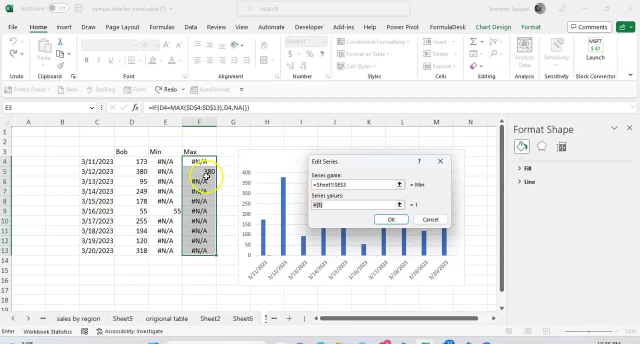 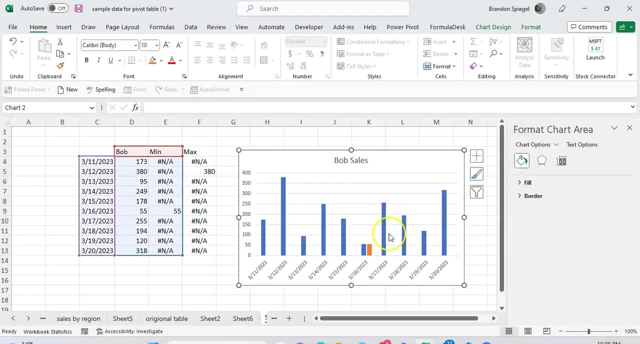 the series name is going to be min, and then the values that represent the series is going to be this right here: Click okay, click okay. and now, as you can see, we have one bar for the minimum and now we're going to do the same thing but for max. so click on the little filter icon. 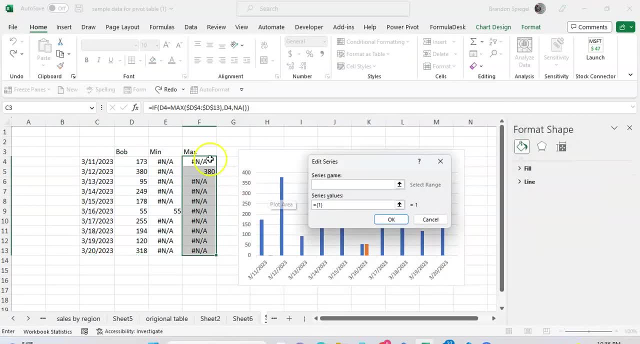 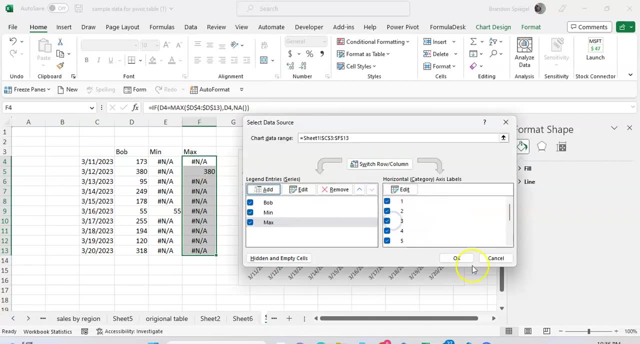 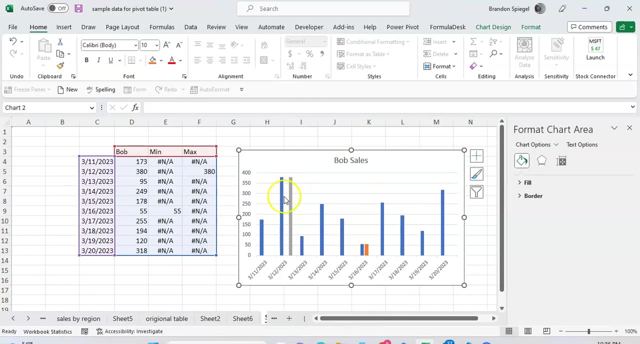 click select data, Click add series name, max And the series values is the values that represent the max. so click okay, click okay, and now we have a clustered bar chart where we have two bars for the maximum and two bars for. 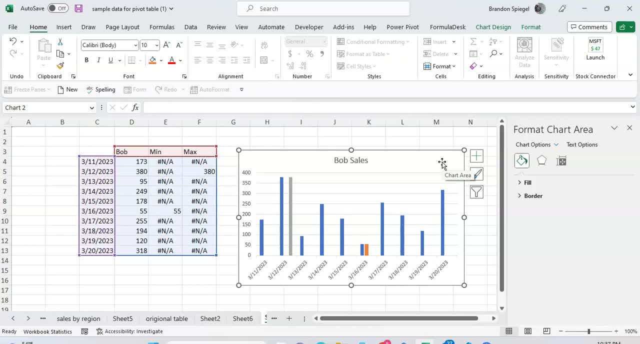 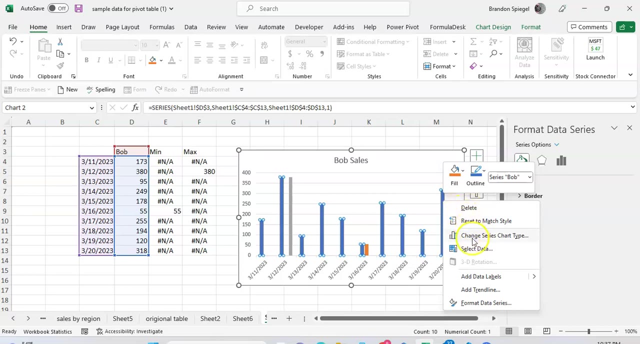 the minimum. So to adjust this so that way we only have one of these two bars showing where applicable, we're going to click on one of the bars to highlight them all. then right click. After right clicking, this little menu will pop up. go to the bottom of it, click format. 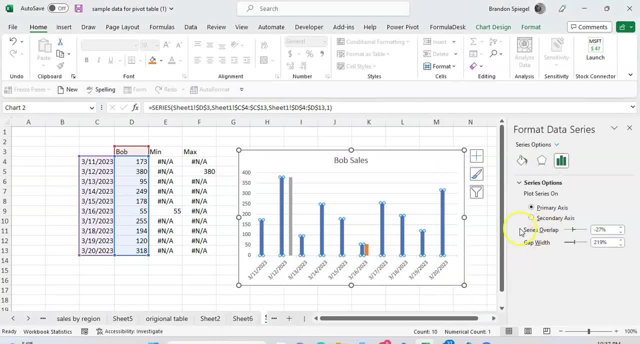 data series and then the magic trick right here is that the series overlaps. as you can see, it overlaps less whenever it goes negative, but we're going to change this to be, all the way, 100% And, as you can see, whenever we do this 100%, the values that were once clustered now completely. 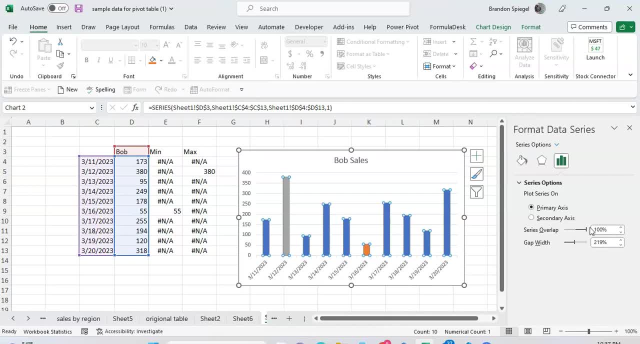 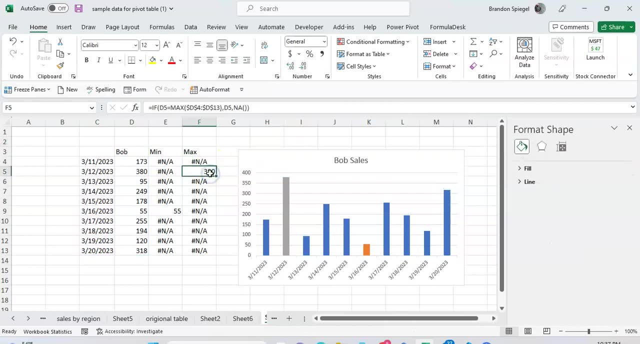 overlap each other, And because the original values are now completely overlapped, we're going to change this to 100%. And because the values that are clustered completely overlap each other, it gives us. and because these are exactly the same, and because this 380 is equal to this 380, for.